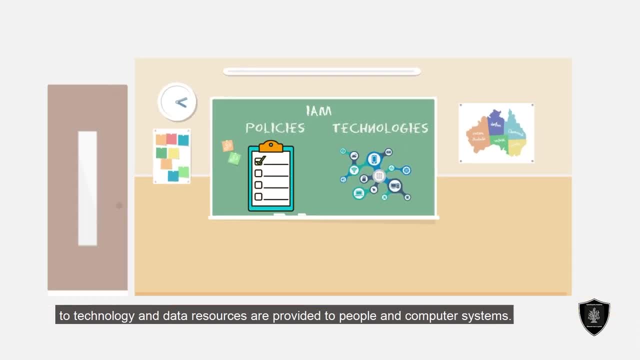 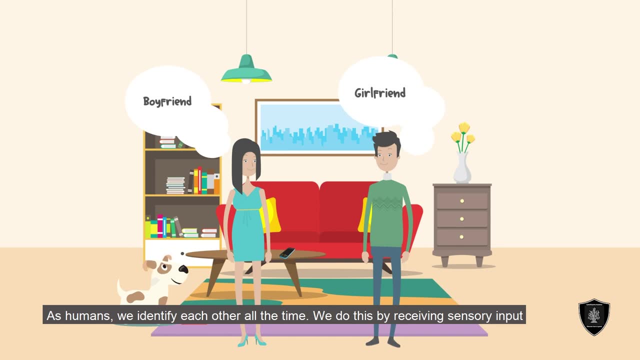 Appropriate access to technology and data resources are provided to people and computer systems. IAM is not a new concept. As humans, we identify each other all the time. We do this by receiving sensory input and then use our brain to process that input. We then identify familiar 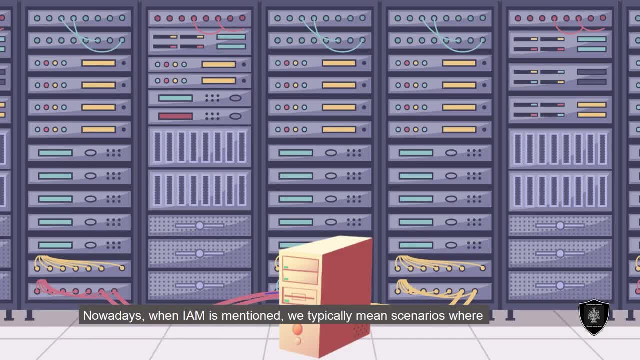 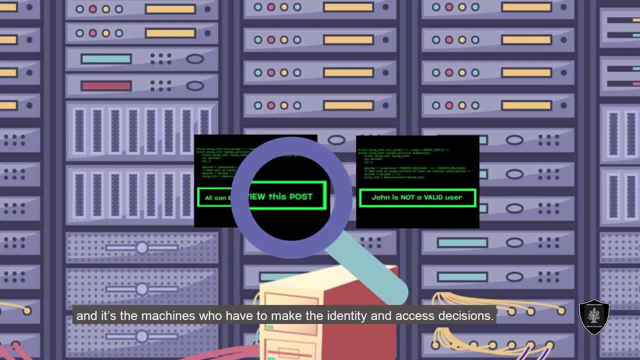 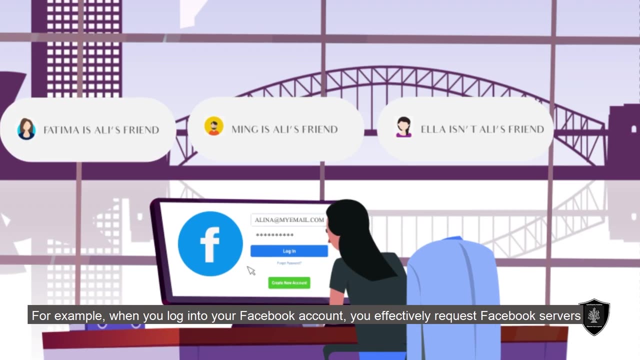 objects and people. Nowadays, when IAM is mentioned, we typically mean scenarios where machines are the recipients of the input and it's the machines who have to make the identity and access decisions. For example, when you log into your Facebook account, you effectively request Facebook servers to validate your access and determine what posts and content you have. 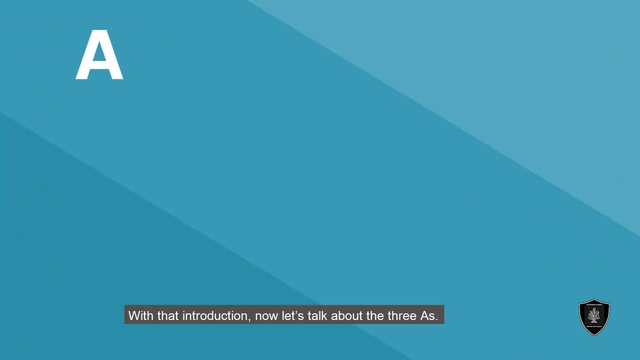 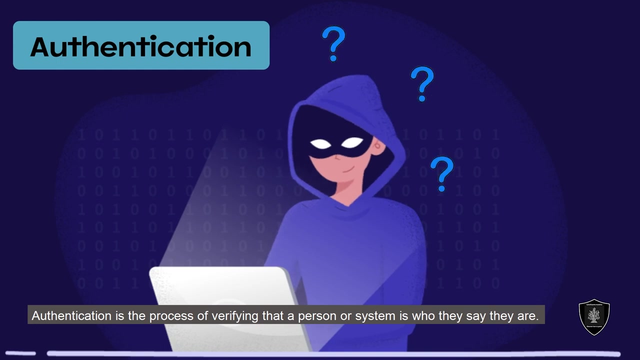 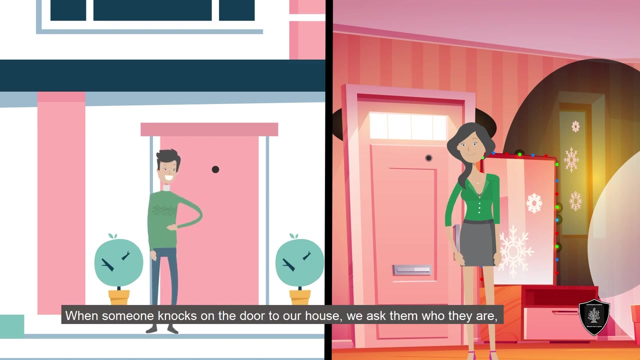 access to With that introduction. now let's talk about the three A's. The three A's are authentication, authorization and accounting. Authentication is the process of verifying that a person or system is who they say they are. Again, we as humans do this on a daily basis. When someone knocks on the door to our house, we ask them. 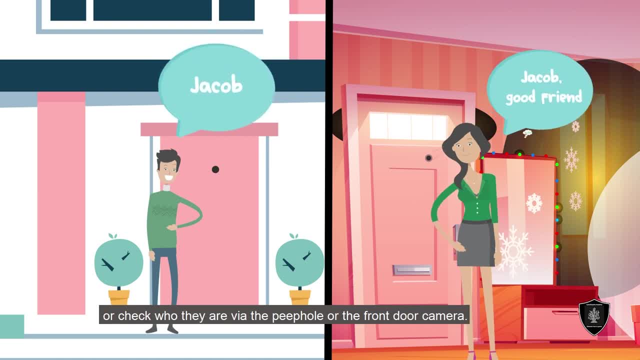 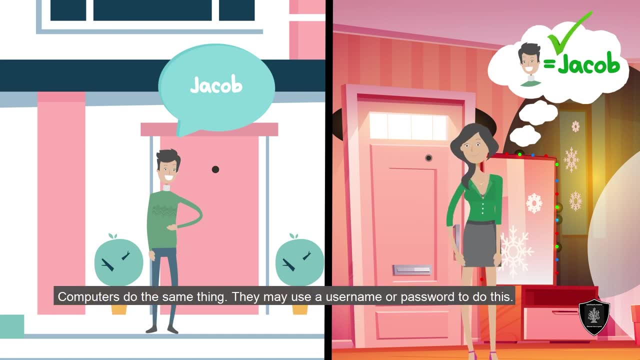 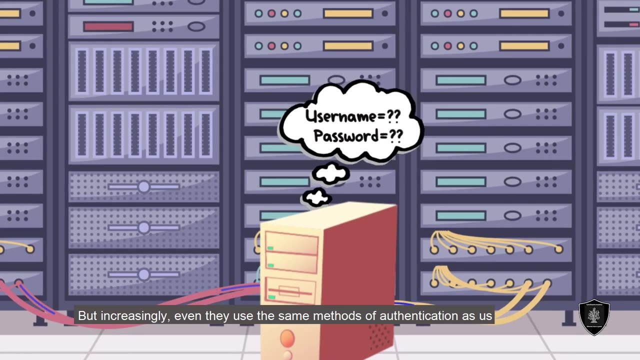 who they are, or check who they are via the peephole or the front door camera. We then use their voice or face, or both, to verify their identity. Computers do the same thing. They may use a username or password to do this, but increasingly, even they use the same methods of authentication as us. 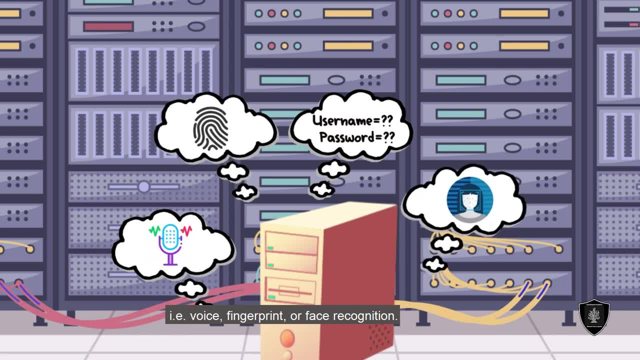 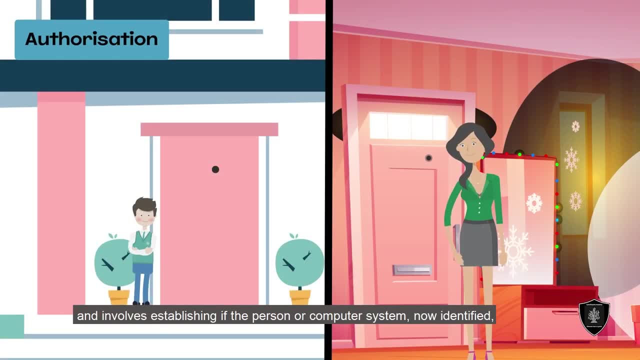 That is, voice, fingerprint and password. The next concept is authorization. this typically happens after authentication and involves establishing if the person or computer system now identified is allowed access to the IT resource or the data they have requested. To go back to our analogy, you may establish who was knocked on your 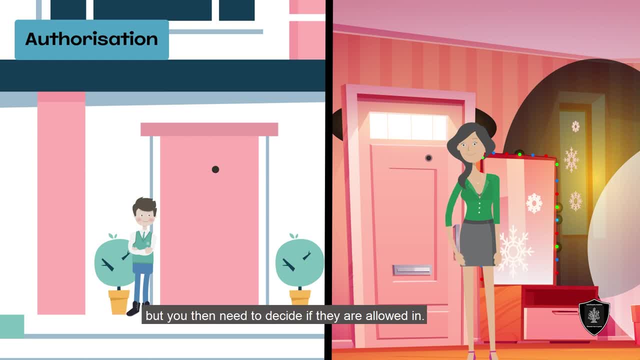 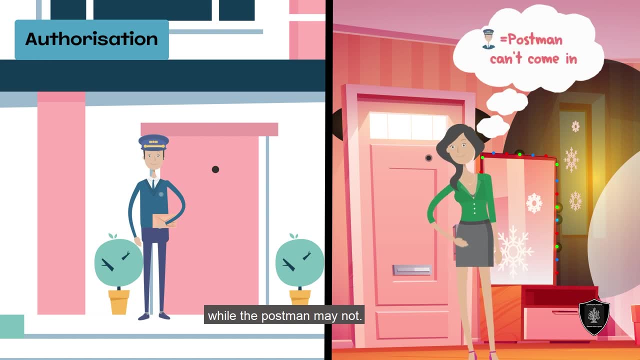 door, but you then need to decide if they are allowed in Your family and friends would be, while the postman may not. For IT solutions, this is done via a database that stores what each person's or system's access rights are. The third A: 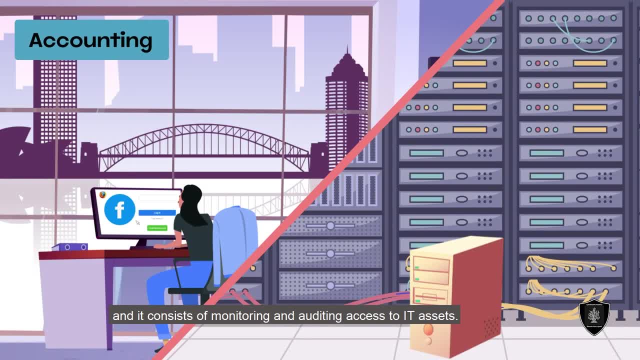 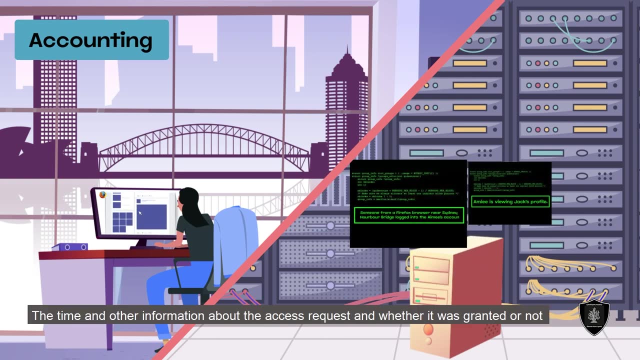 stands for accounting, and it consists of monitoring and auditing access to IT assets. This gives us the ability to capture and review the systems that have been accessed, persons or systems, who requested access, the time and other information about the access request and whether it was granted or not. In our